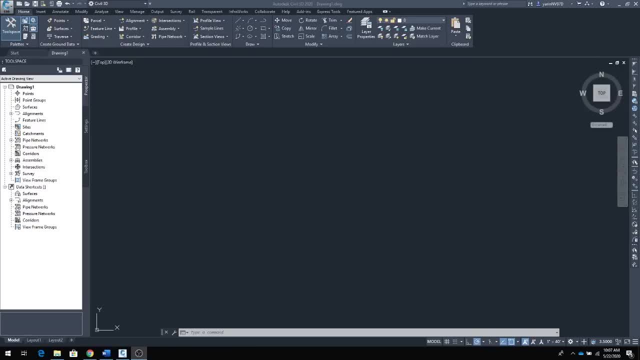 We're going to work with the CivilCAD 3D and do some basic highway design sketching. First we're going to start out to importing some data and then we're going to go ahead and create a surface and then create an alignment profile and get to a sections and a corridor. 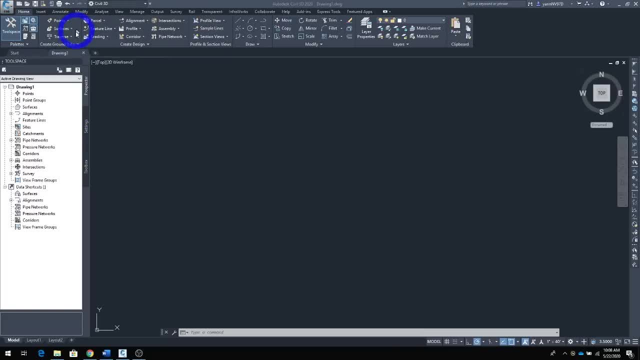 So one of the first thing we're going to do, we're going to import data, whether it would be a survey data or a point file. So let's go start with a point file, and we're going to click on a point right here and this new window open up. 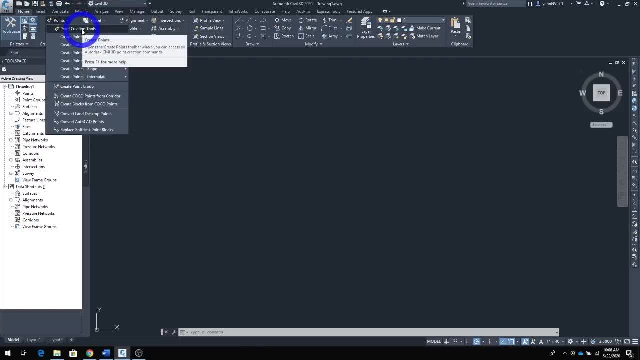 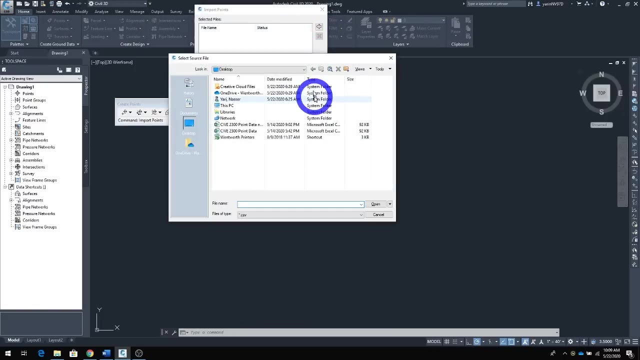 It says point creation. click point creation and then you see another window open up In this window right here. click this import file and then another window open up Right here. you see this plus sign. click the plus sign. That will take you to your. make sure your file is on your computer, not on a cloud. 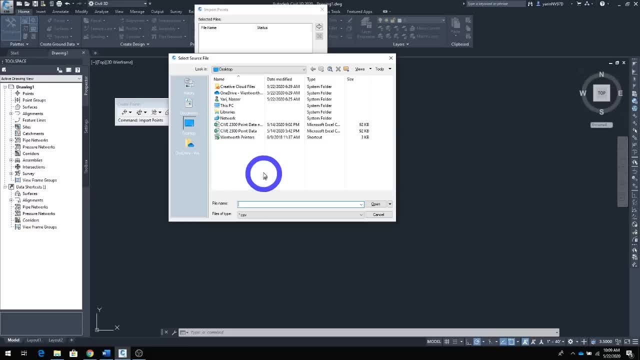 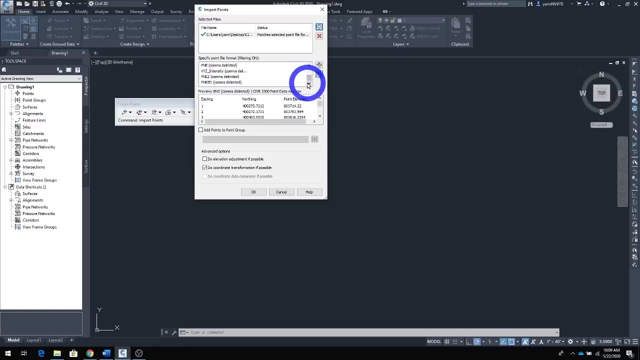 And once you're here You can pick up your file. Let's see if we can find that. Here we go, And once you click the file, you go through your file, take a look at it And in this second window, go down here. 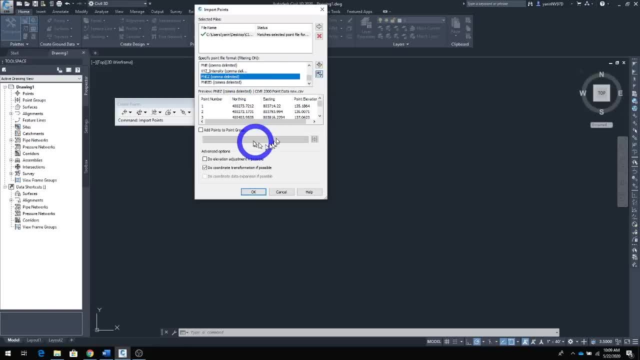 There's something called PNEZ. Click on that and make sure everything is in order: Northern, Eastern and point elevation. That looks good. And down here, make sure this one is checked and the other two are unchecked, So you do not do coordinate transfer, if possible. 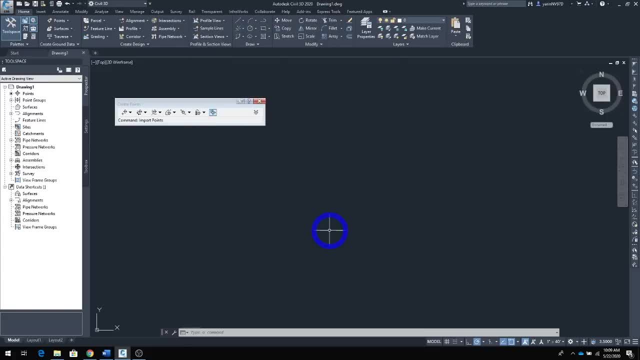 Once you have that, click OK. And then you click OK, You now you look at your screen. you see nothing. It's OK, Don't panic And go ahead right. in this You can do two things. One: you can type in: zoom, enter, de-enter or just go over right here. 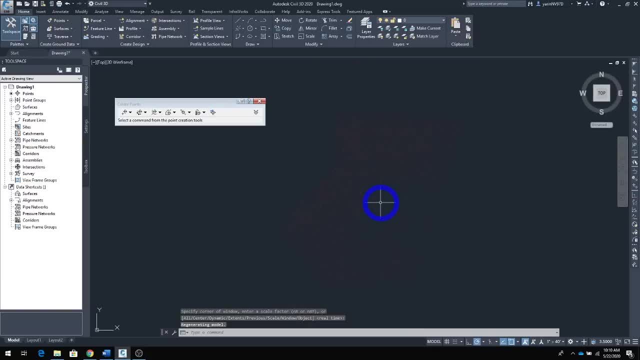 Right, It says zoom, extend. Click on that, And there you see your point data. So next thing we're going to do, We're going to go: Go to the next one. Go to the next one, Go ahead and create a surface right from your home tab. 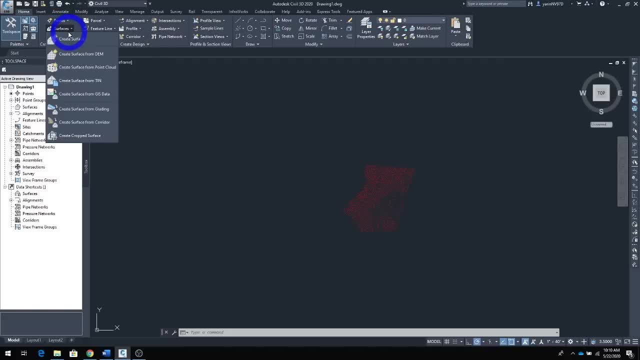 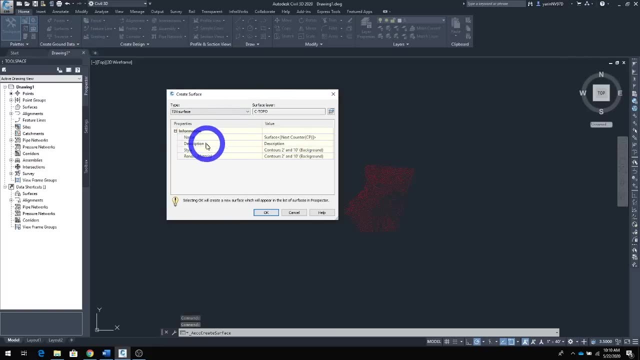 Go to surface and click the drop down menu and you see: create surface. Click that, Then you have this new window open up. Let's name this surface the name the surface because it's the existing ground. So we're going to call it W-I-T-E-G and now we have that. 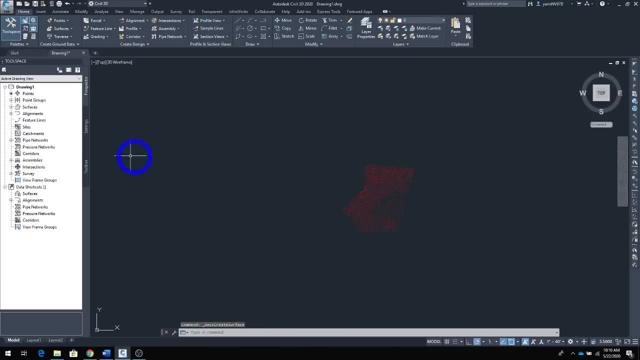 We're going to click OK and going back to the prospector, They call this a prospector. This prospector you can. if you click on that tool space right here, it's gone And if you click it's back on. 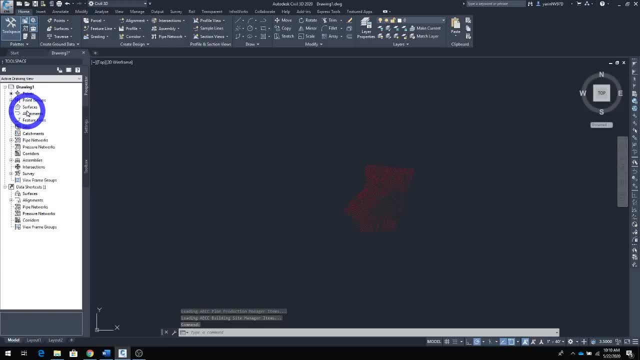 So we go to the prospector and you find the surface. When you look at the surface, right next to it is a plus sign. Click that plus sign And after you click the plus sign, look down. we see the file that we created called W-I-T-E-G. 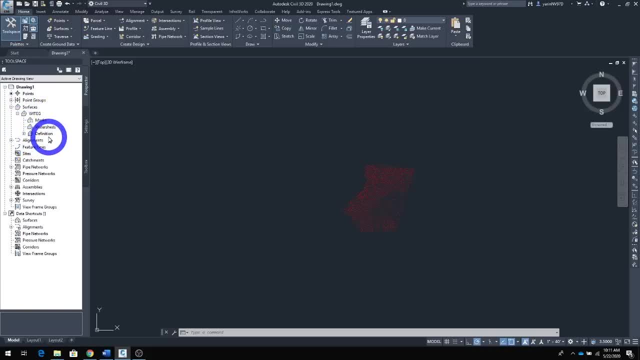 Click the plus sign on that also, And then you go down. you see a definition and there's a plus sign next to it. Click the plus sign next to it And we get to where you see this opens up and you go down here. 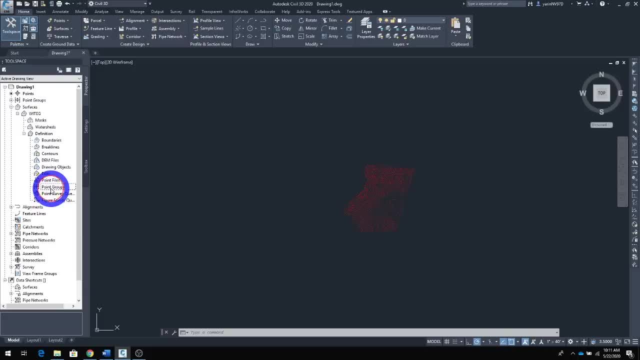 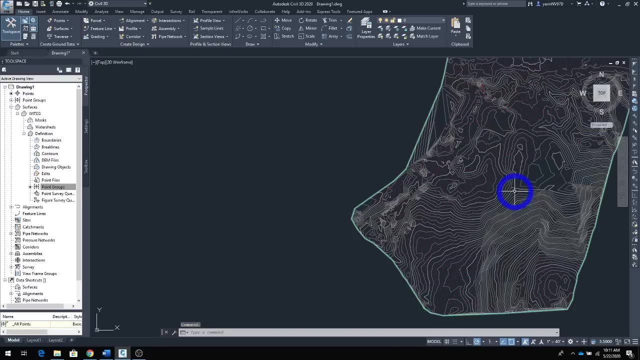 What do you see? It calls a point group. Click on a point group and then right click your mouse and you see this says add, Click, add, And when you click add, a new window open up and click all points apply. OK, so now we have our surface created. 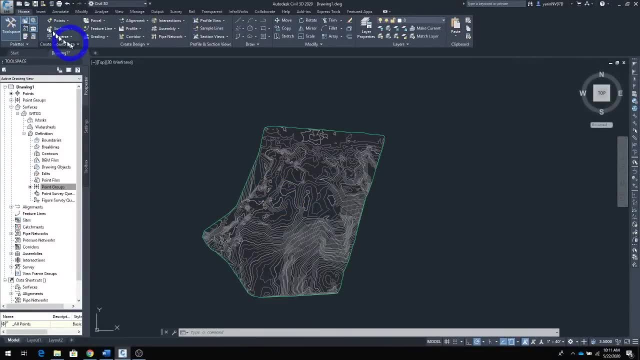 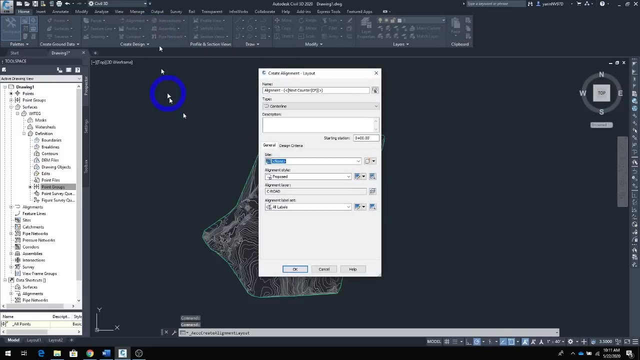 From here we're going to go ahead back to go back to the home tab and go to alignment. Let's make the alignment and you can see right here we have alignment. Click on alignment and alignment creation tool. OK, let's do that. 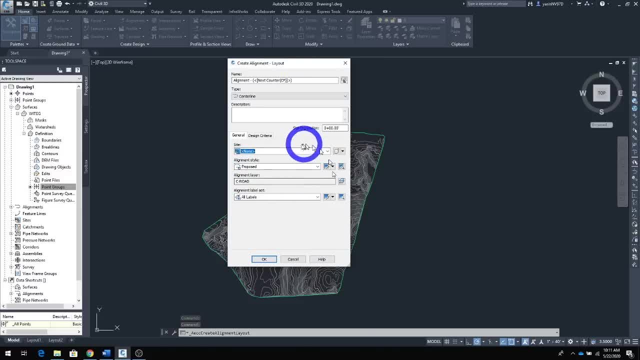 And then this new window opens up right here And there's a lot of good information in here. Let's name the alignment first. OK, just let's call it alignment W-I-T And come down here. It says This side, leave it where it is and leave this window proposed. 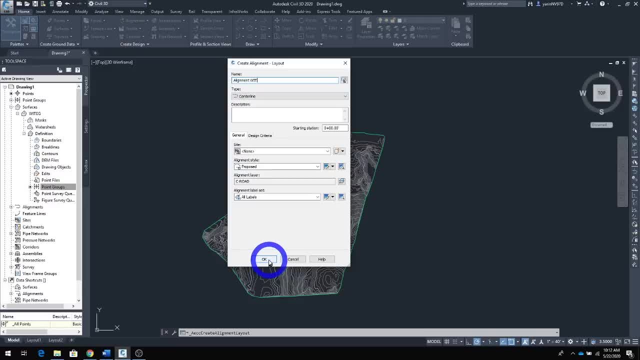 That's fine. All labels? That's fine. Let's click OK And starting right here is a staffing station: zero plus zero And you see this is general If you go design criteria. they got the code in here. Minimum radius table from AASHTO. 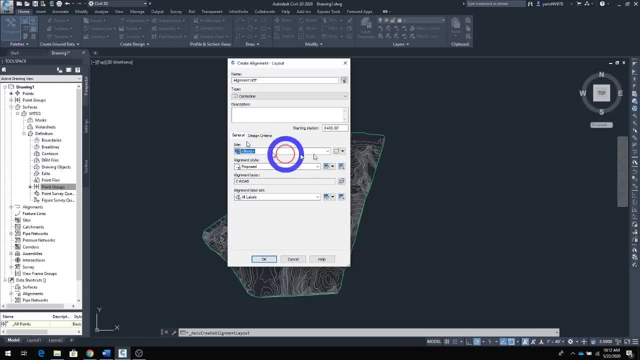 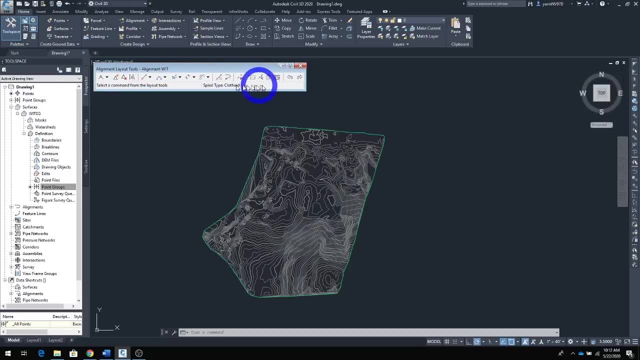 This thing is amazing. So now let's just go back to the general and click the way they were. So click, OK. And when you do that, this new sketching tool kind of opens up on top here. From here you can go to the far left and you see this. click that drop down menu. 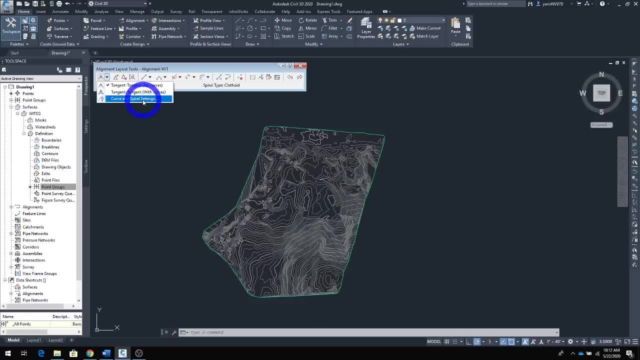 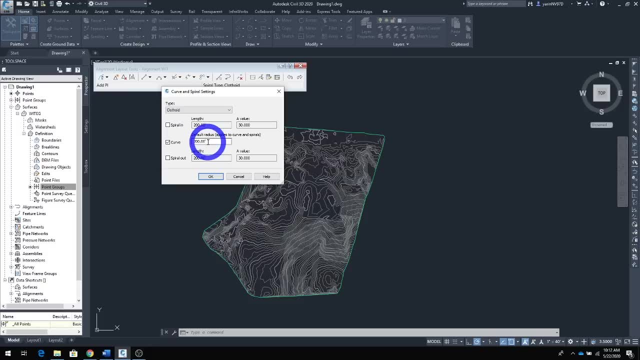 And down here is a curve and spiral setting. You click that and this new window open up. It says: view on your curve Curve will be 200.. You can switch that based on the code you're using. So leave it the way it is and click OK. 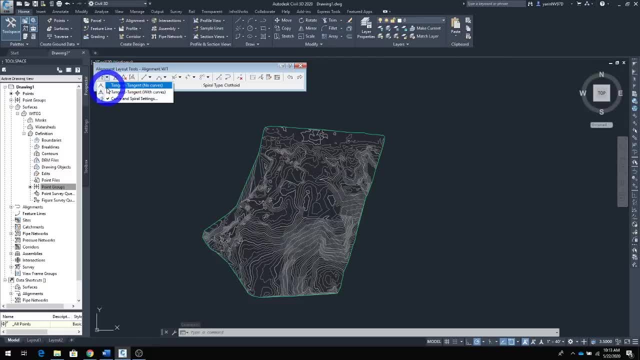 Go back again here, Same drop down menu, And you have an option, The option pick the tangent to tangent with curve, And once you do that, now you can draw your profile from this point to that point. Let me make this a little bigger. 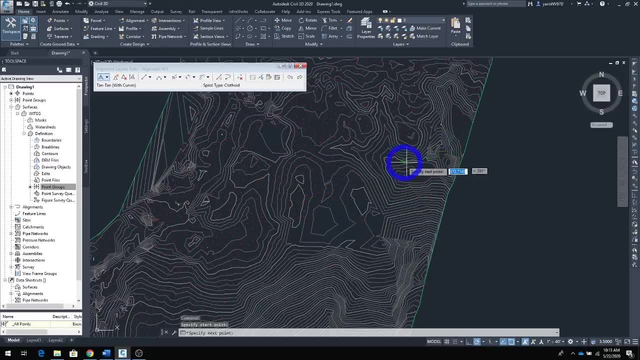 There you go. I'm going to start from this point right here, and click right here and stop right here. Just click it and then take a curve right here and click down on here and come back. this way, Let's put another curve in there. 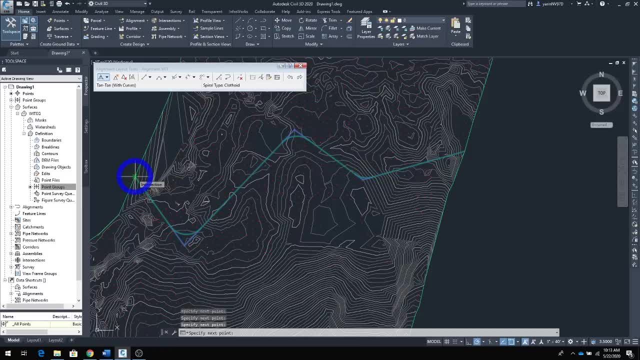 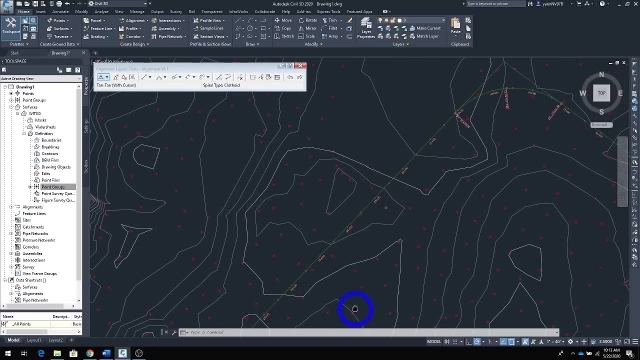 There we go, Click good, So now we're done. And then, once you get to this point, click enter All right, And you see, right here you created the alignment and you see the stationing. And if you come back down, we made that turn the corner. 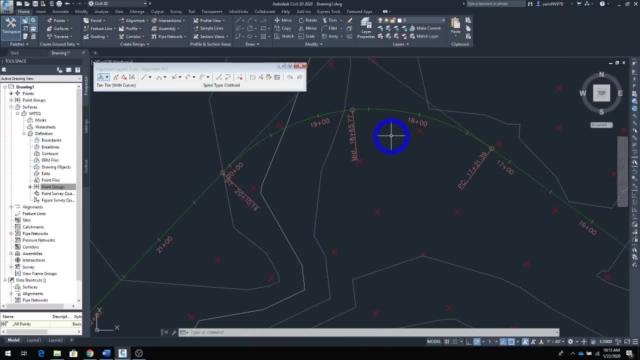 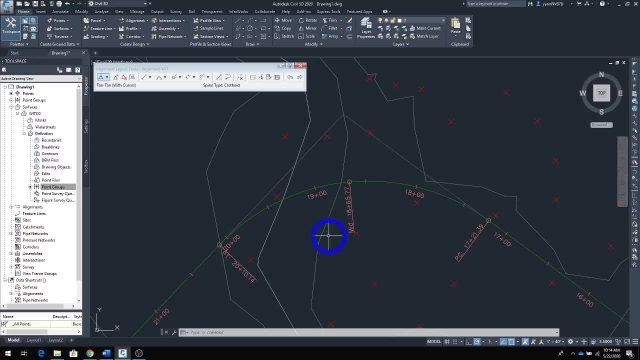 We made a horizontal curve right here And we look at the. you see the horizontal curve data. You have your PC, you have your PT and your vertex right there. This is amazing. This already does that stuff for you. Okay, So now we sit here. 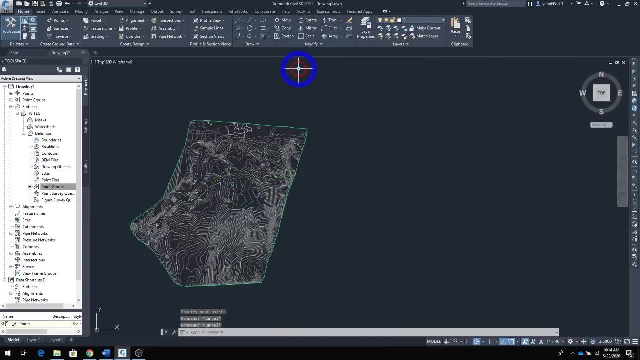 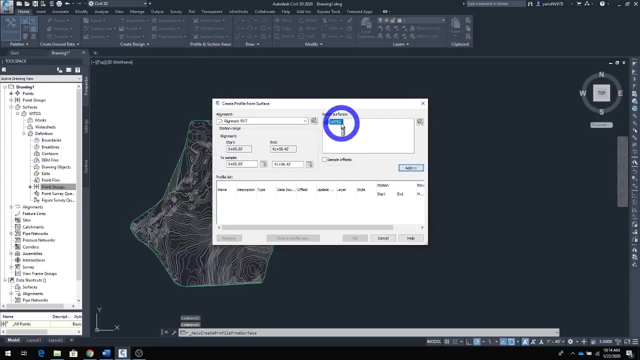 We created the alignment, Let's go ahead, create a profile. So go back to the home tab. right under alignment There's a profile. Click the profile and it says create a surface profile. We click that new window open up. It says okay, you want to go from the WTEG existing ground alignment. 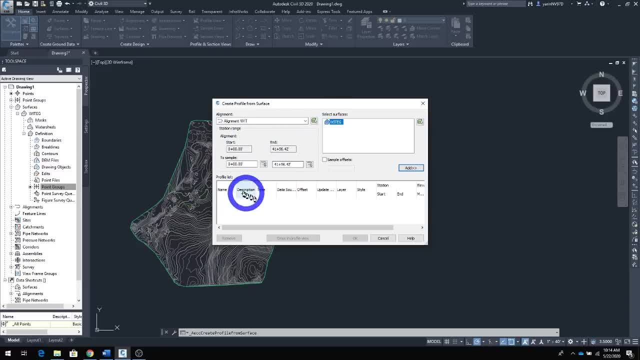 It says yes, From station zero to station 41. Yes, That's what we want to do. We click add And when you click add, this window opens up down here It has some other option, But from here you really want to go ahead? click draw in profile view. 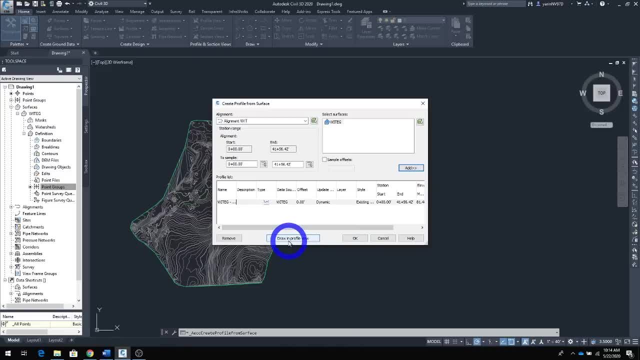 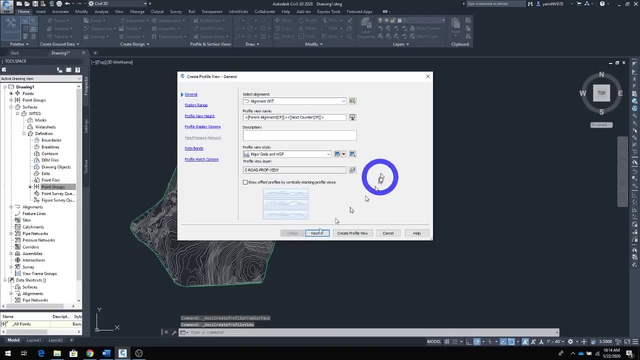 And if you hit okay, then you have to come back again to this point and view file. to draw in profile view, Let's click here. And once we click this, this new window opens up And in this window, basically it goes through all these options, from general all the way to the profile setting. 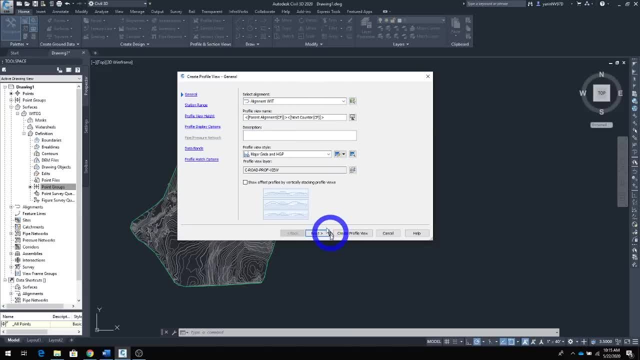 So it says: hit next when you get to this window, and it talks about the alignment: Yes, this is the alignment we want to do. And then it talks about what stationing if we use it. we have an option- automatic, or we use our own. 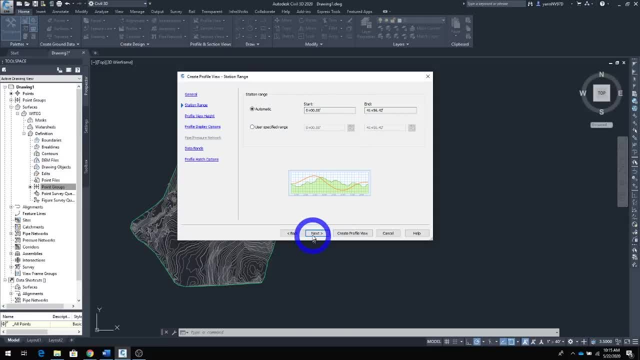 Let's go with automatic from station zero to station 41. We click next the same thing option with this elevation, which is going to start from 81 to elevation 108, or you can use your own, But let's go with automatic again. 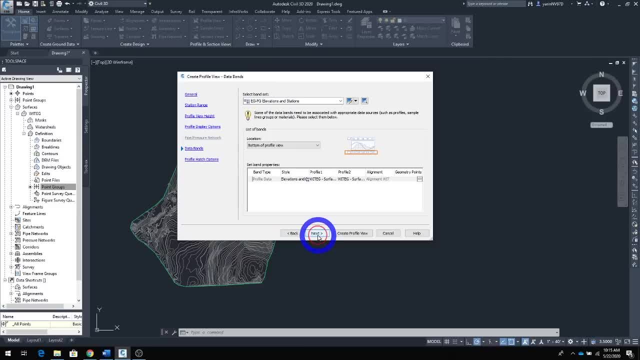 Click next. When you come to this window, again click next one more time and it clicks another time. Click next, Go through all the stuff And finally, here, when you get to this window, click create profile view. Now you notice, when you did this, you come to here. 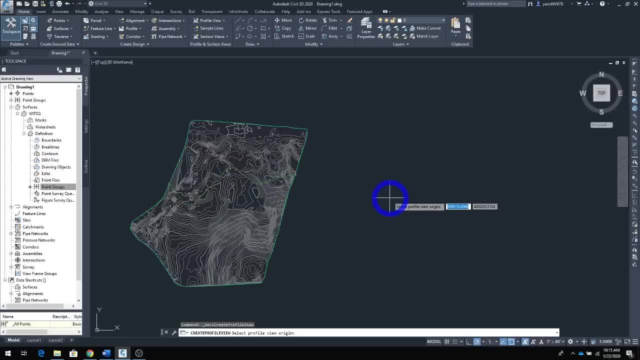 It's like: where's my profile? Relax, See this. It tells you where you want the profile. So go right, Find a spot that you want to write here and then click on the screen and there's your profile view. So now you look at the profile view. 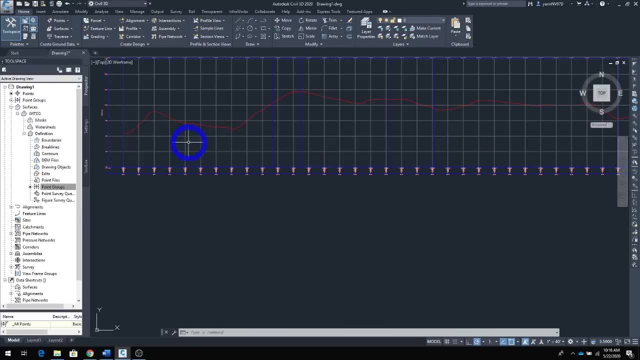 You can see it, and it's a good existing profile. It's a good place for doing either for wheel or motorcycle. but we don't want to do that. We want to put a new profile, new road with a good slope to it. 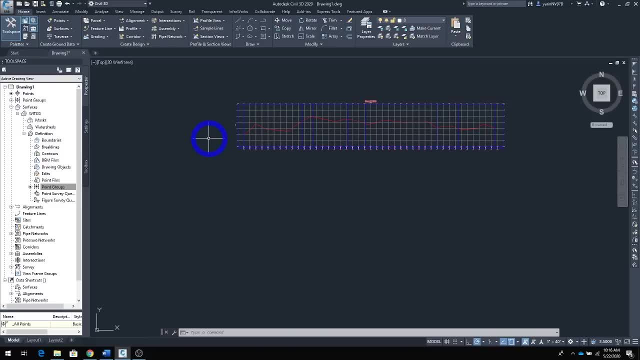 So let's go ahead and create a new profile. So while we're here, we go back again from the home tab. We go to profile right here and it says profile creation tool. We click that one And once you do that, you come in. you see, your mouse has a little square. 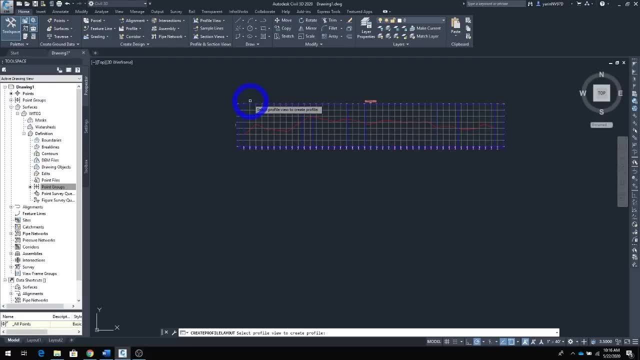 in the middle of it. so hover that square over your profile when it lights up. See, it lights up and you go once it lights up right there. You got to make sure it lights up right there. Okay, now click it, And then this window comes up. 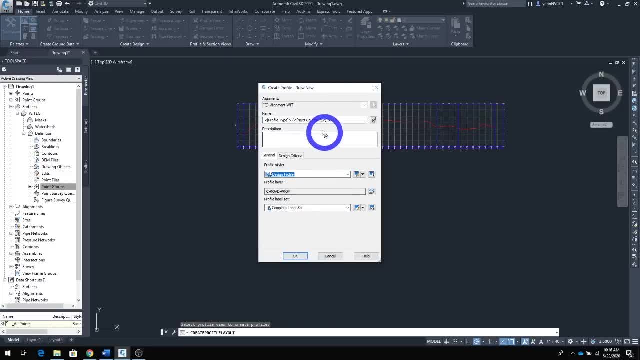 When this window comes up, you want to fill all this information. It starts out with alignment WIT: Yes, Name the profile. We're going to name it right here, So we're going to say this profile name. This is our second one. 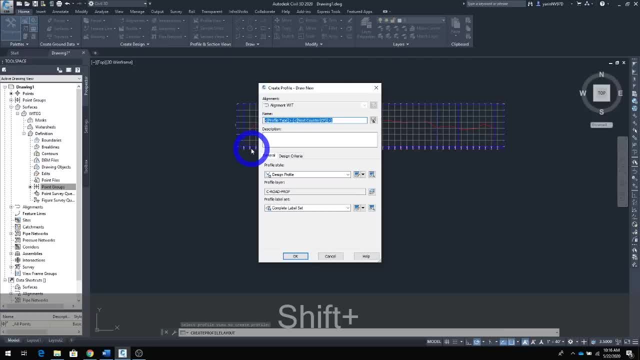 We made one for the existing, So this is going to be for the new one. We're going to be WITFG for finish grade or finish ground. So now we have this and they have design criteria, all that stuff. So design profile. 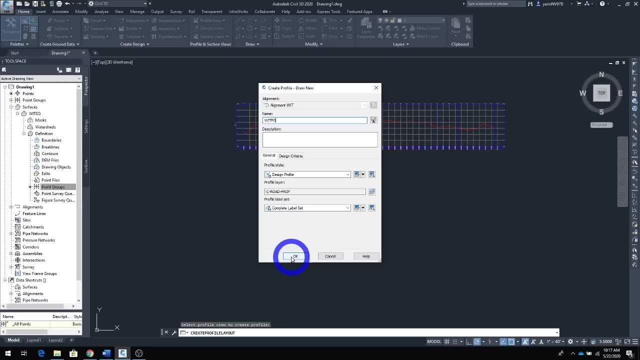 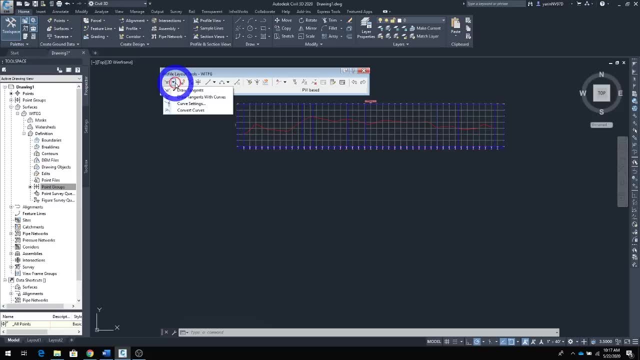 Correct, Complete, set a label. Let's click Okay, Again, we end up with this sketch tool. We do the same thing over here. Let's go to the curve setting and look at the curve setting and horizontal. You have a horizontal curve. 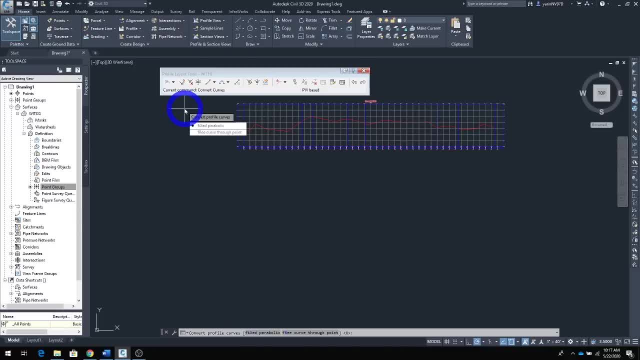 I mean an alignment. You have horizontal curve and then profile, You have a vertical curve. What happened here? Let's do that again. Curve setting- Okay, Now we go back to the curve setting. They have all the value here. 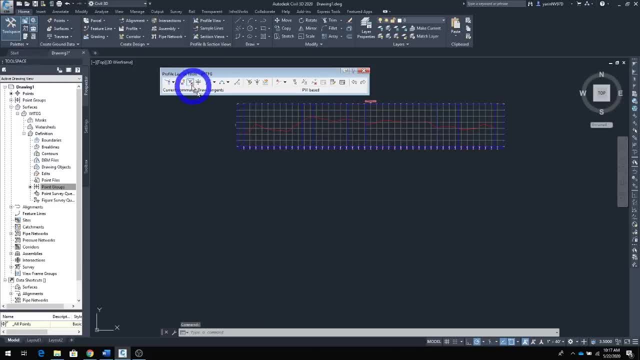 You can leave it the way it is for now and click Okay And we go back to a curve draw tangent with curve, Same thing, And now we can do our drawing. Let me make this a little bigger. Okay, I'm going to start from this point here. 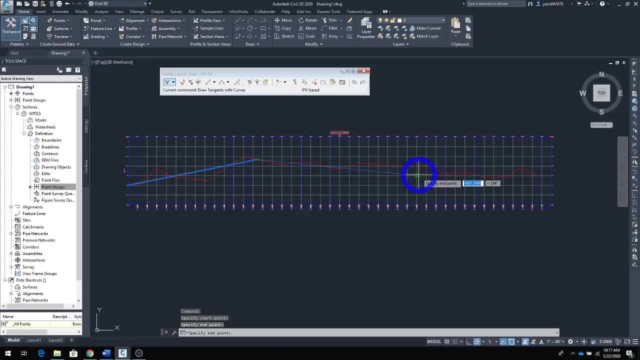 I'm going to go up right here, Come back down here, Put some couple of vertical curve in it and finish it up Right Here, And once you do click enter and there is your profile, Let's see what you got for grid here for elevation slope. 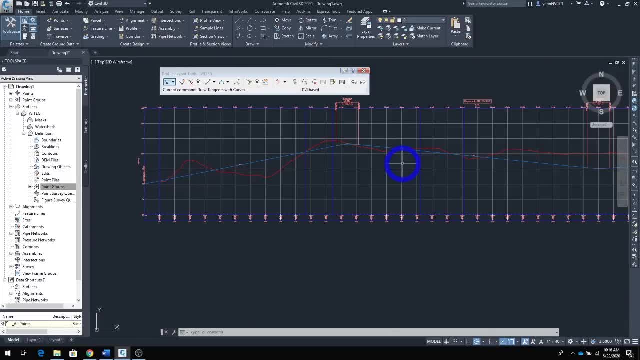 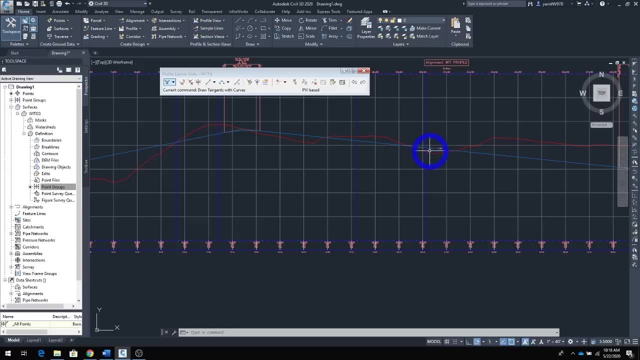 Right, There's a 2%. That's pretty good, And you got 1.1 minus 1.0%. The one thing is you want to stay at around half a percent and between half a percent and 7%. you don't want them to flat. and then you want to steep. 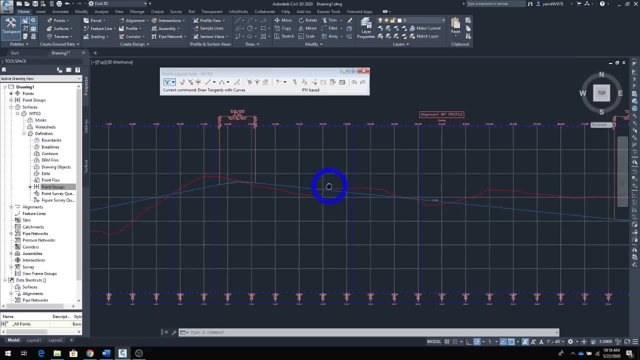 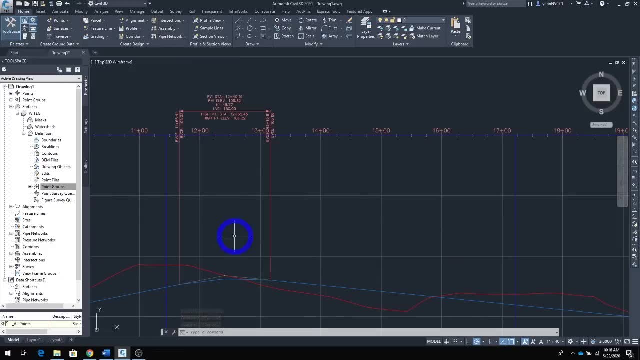 Either. now we have this, and let's check something else out. If we get rid of this, here you can see the curve data for a vertical curve data. It's way up here, way up here. Let's bring it down closer to our curve itself. 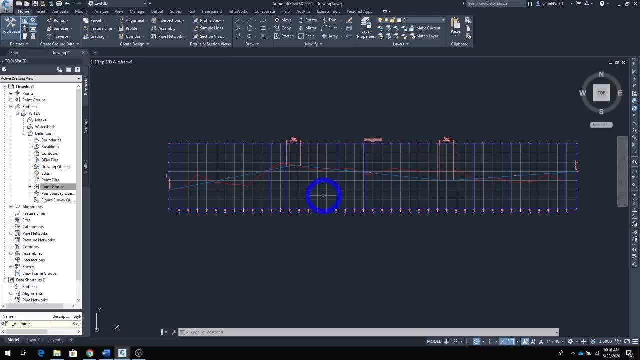 One thing we can do: go on your new profile right here and you can see when light up. See if you go back right on top of it and click the mouse and now you have everything is light up from rare. This program is amazing. It's so smart. 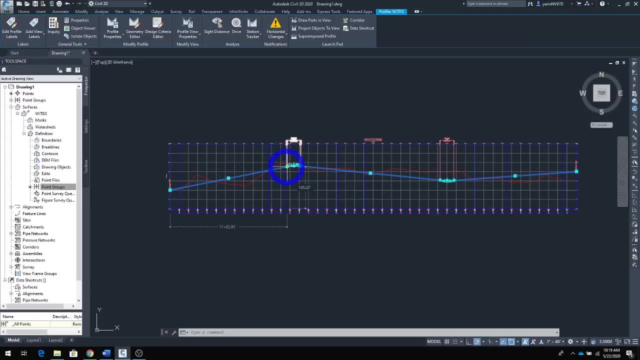 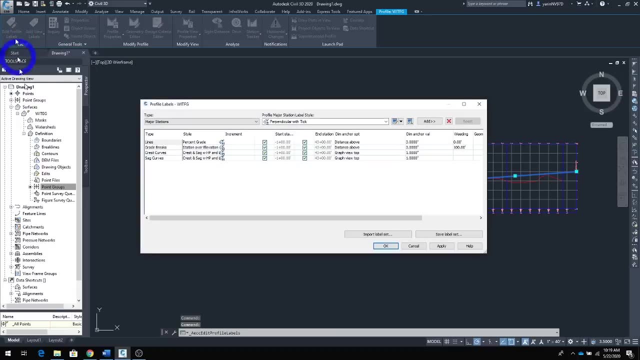 That's everything for you. So now you clicked on this and it's highlighted, You go up in a ribbon. in a ribbon in the far left corner, You said it says edit profile label. Click that and then here, tell you about your labeling. 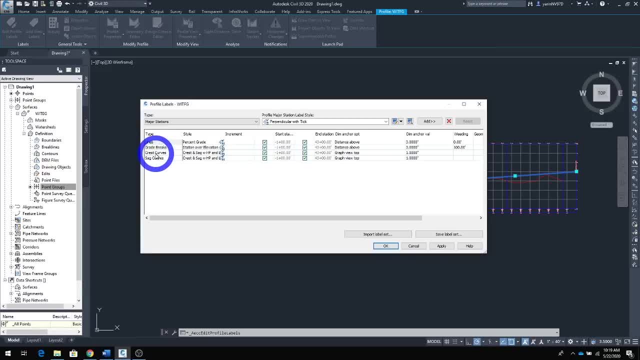 So you go to right here, crest the curve and sag view and you go all the way across. It says: okay, grab a view on top, Click on that and click one more time and you can see the drop down. It says the distance above. 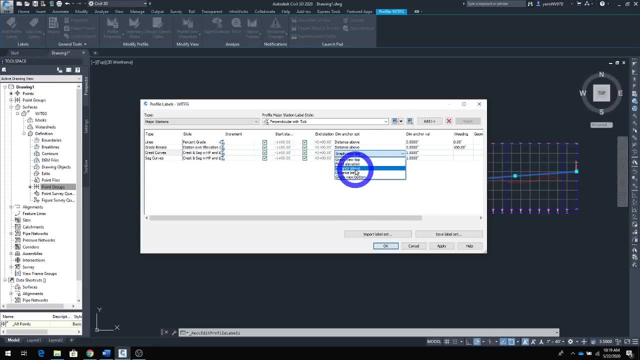 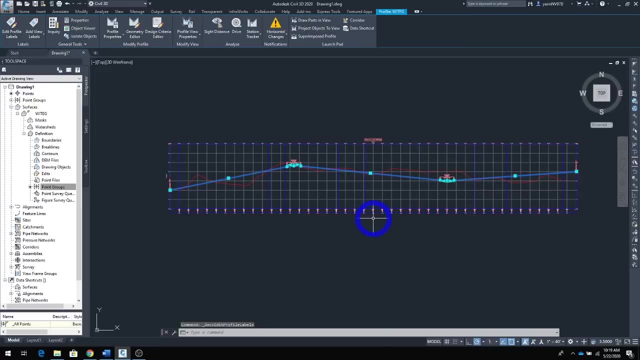 Let's make a distance above Or you can choose whatever you want. So I'm going to go distance above. I will do the same thing for the one blower, for the sag curve and distance above. There we go, And here how much distance above is, type in one inch one and enter, and you will see it didn't work. 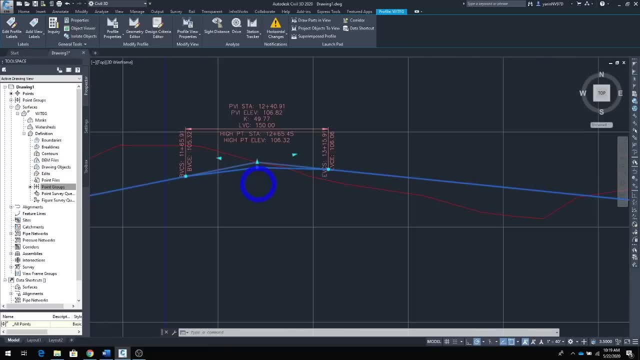 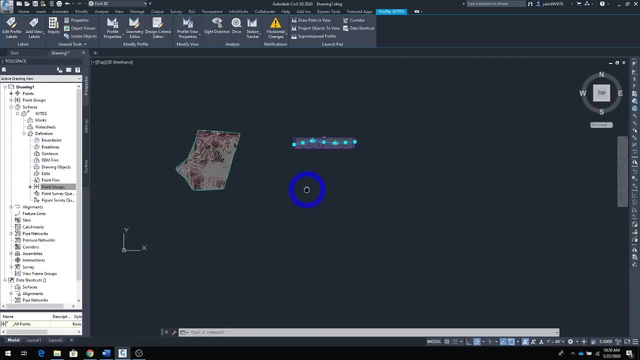 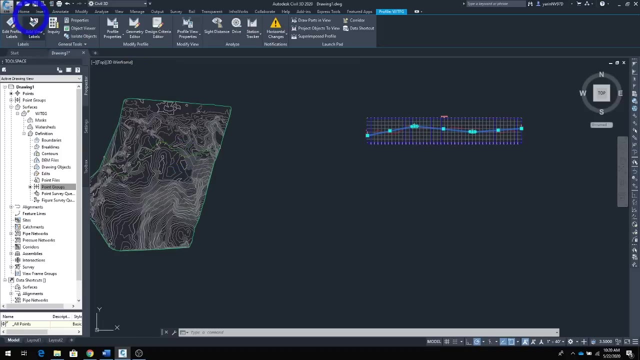 Okay, right here, There we go. We got it. We got it down here anyway. So now we do this and let's do something else, and that is do the typical section, or what we call assembly here. So go back to the home tab, right here. 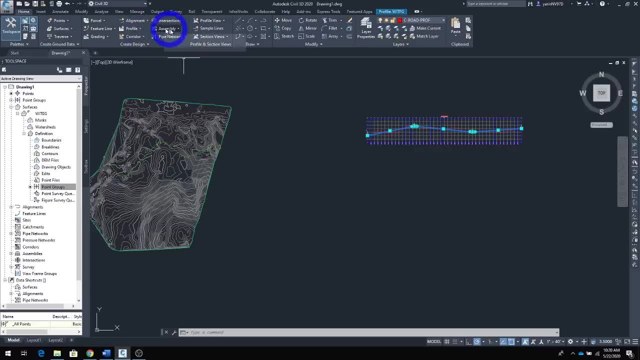 And there's something right next to the profile over call assembly. Click that assembly tool right there and it says create assembly. So when you do that and you have come to this window, just fill this window up. Name of the assembly You can call it. 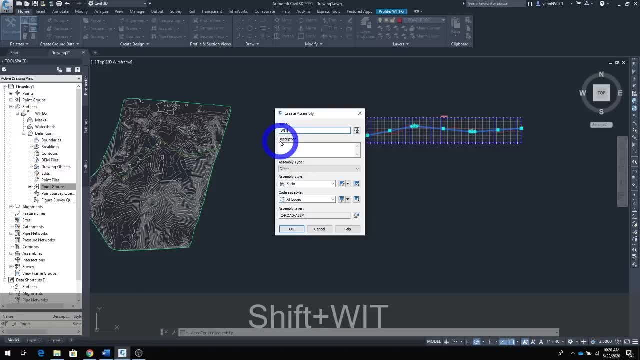 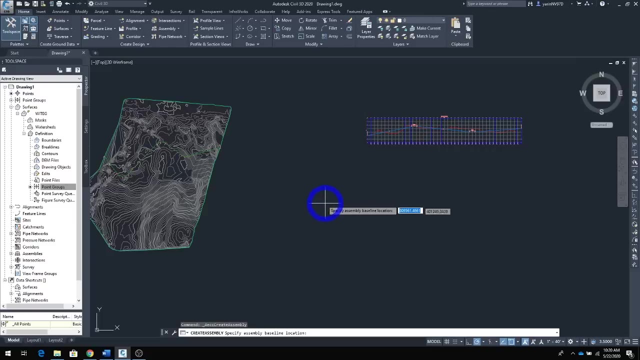 I don't know W A T One for now. And then you come back here: The basic is good and all code, And let's go click. Okay, And where do you want it? Now? that's what the mouse says. 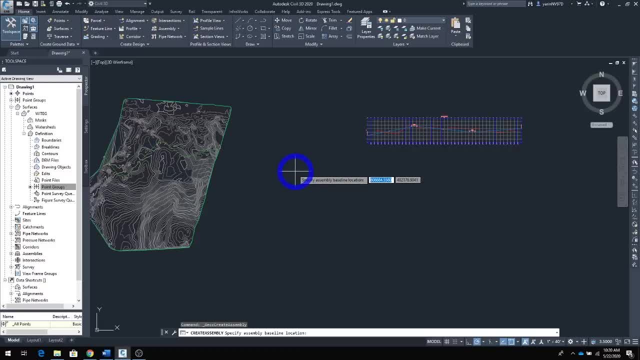 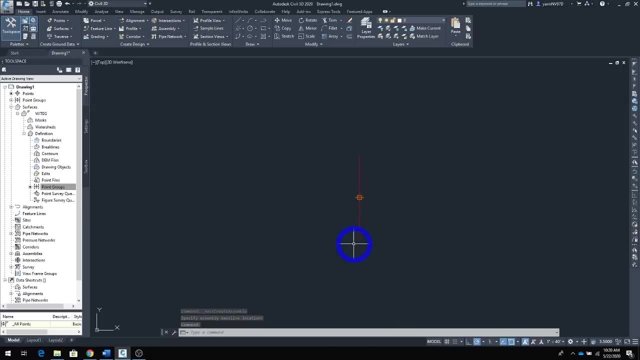 Where do you want this? Let's put it right here, between both of them, Right between both of them, And notice that like this. So you see right here. But this is very small compared to our alignment and profile. Let's zoom back in. 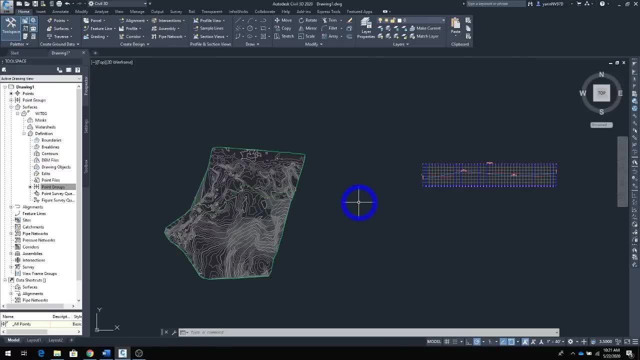 It is. see how small you see that red dot like that. That's what it is. So let's move back out and get it opened up. There we are Now we have. Okay, We can work with this. So from here on, what we got to do is go up. 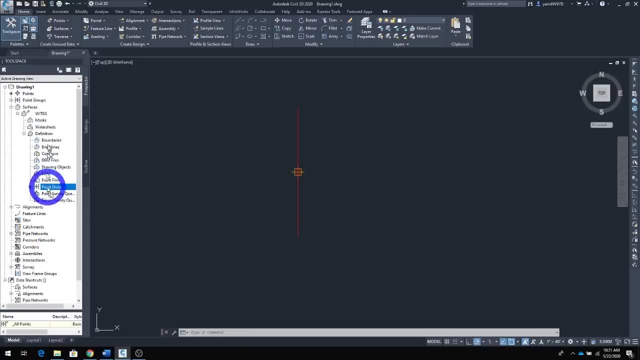 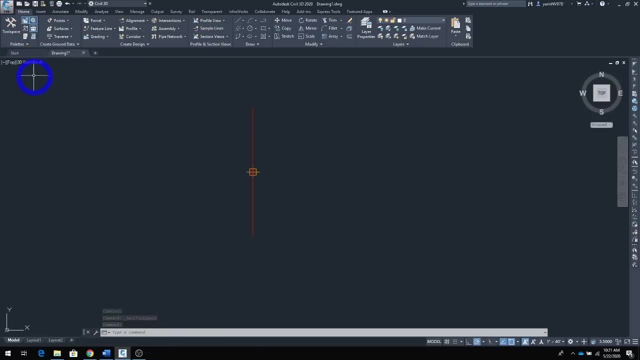 Let's get rid of this prospector. We need a space here, So we click right here. That goes in. If you click it, It will come back again And we want to hit this tool right here, Right there, Right below it. 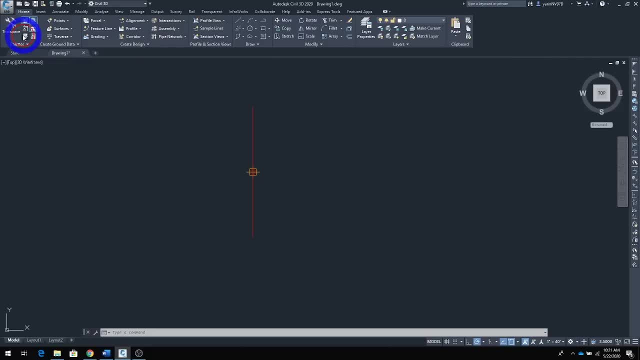 It says, right there, Got it Okay. And when we click that tool then we click the next one next to it with the property. So we click that palette and right here Click this one called properties next to it, And now we have both of them. 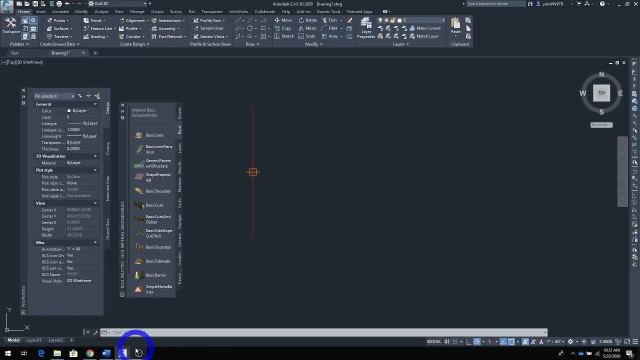 Property and this one is a tool palette. So we click the tool palette in here and then we have the property right here. So when you look at the tool palette right here, it's just amazing. They got so much good stuff in here. 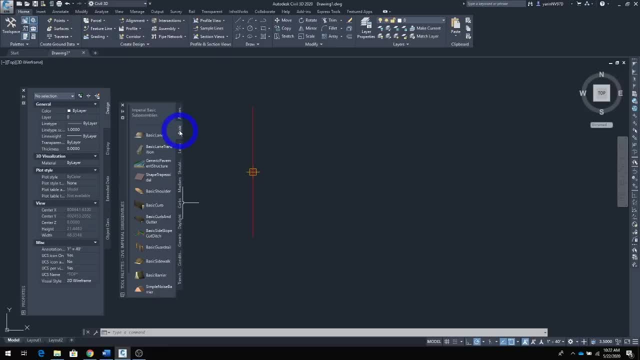 And you see all these different tabs right here. Let's just stay on a basic tab. You can go later on. Go ahead and just explore all these different options. Now, from the basic tab, you can click on basic, All right, And then you come down here. 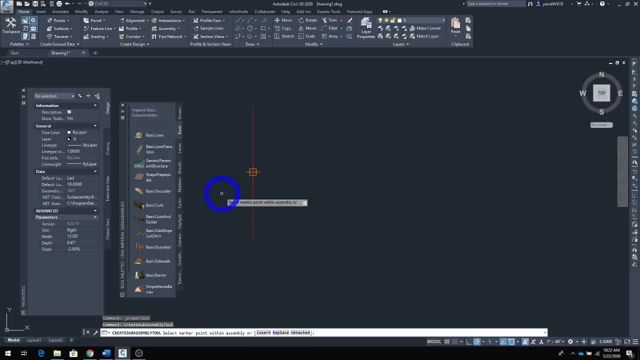 They have a basic Basic lane as we can find that basic lane And when you click that, this other window in the property shows you the basic lane And right here it says the side, right side. That means we're going to work on the right side of our section, right here. 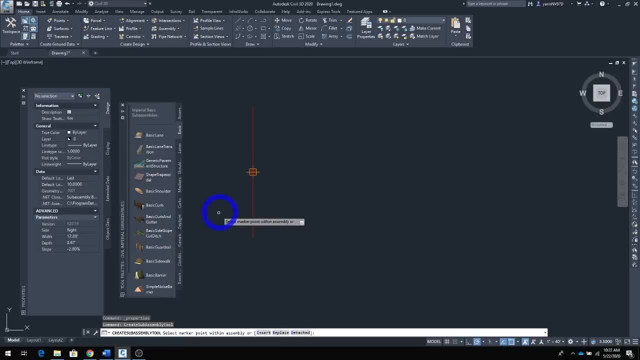 And then the width of our lane is 12 foot lane. That's good, We like that. The depth of our lane, the depth, Our depth really is. the depth is from the finished grade to subgrade. What I mean by finished grade to subgrade I'll show you in a minute. 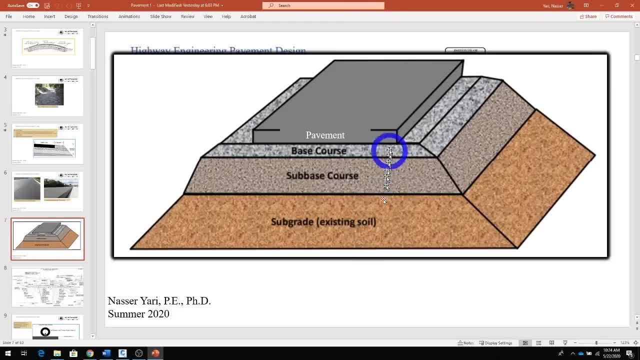 So the depth they're talking about is depth from the top of the pavement all the way to the subgrade- And it's right here- to the subgrade. So subgrade is existing soil. It could be clay, natural material, what's in the ground? 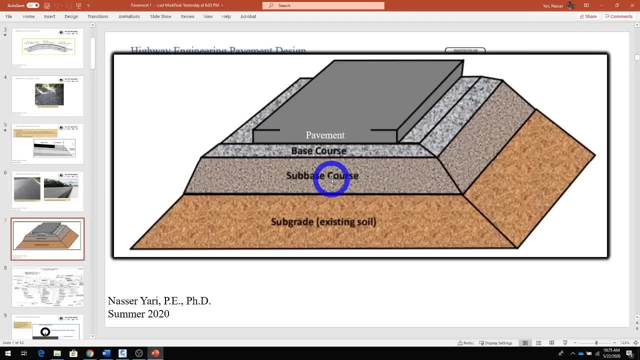 And above the subgrade, we have the selected material. It could be sand, gravel, crash gravel, And then you have the base course underneath the pavement could be nice, clean, crash stone and then you have the pavement And, of course, pavement itself could be a different layer, could be base layer. 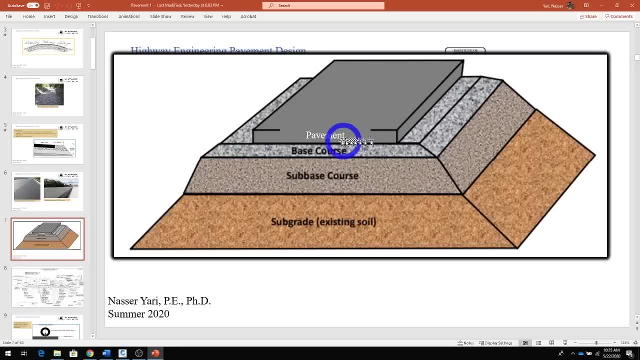 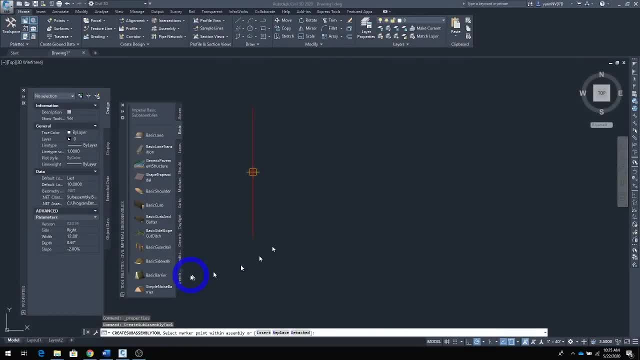 a binder and then finally, the wearing surface. So that's what you're talking about. Let's go back to our drawing. So now, here it says 0.67.. That's really not enough. Let's make that one and a half for now. 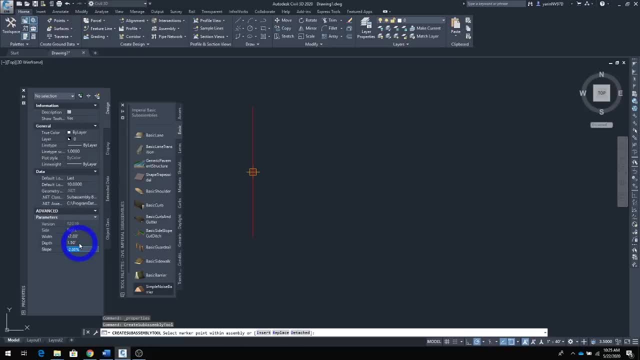 1.5 and click enter And now we have that set. 2% is good. That means from the center line of the road We have 2% cross slope. So we click Okay And we're going to come back in here. 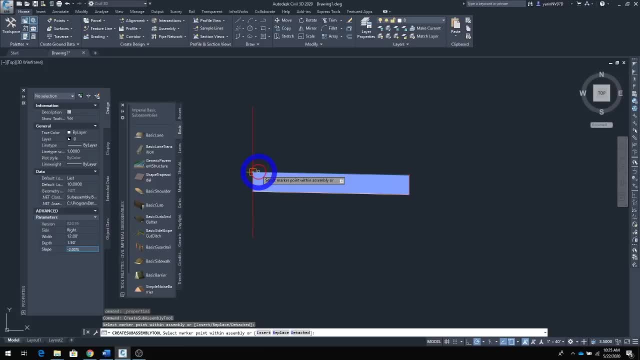 Right here where we have the plus sign right there, Click that and we see our lane. This is our lane And this is our tour for lane. Let's add some shoulder to it And you go in here. you have all kind of options. 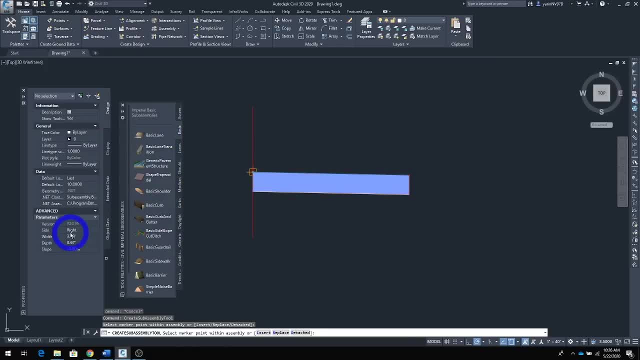 This is the basic shoulder right there. So I click basic shoulder, It's on the right side. Yes, With three feet, Let's make it six feet. Six feet Enter And then depth: Make it one feet Enter And slope is 4% is good. 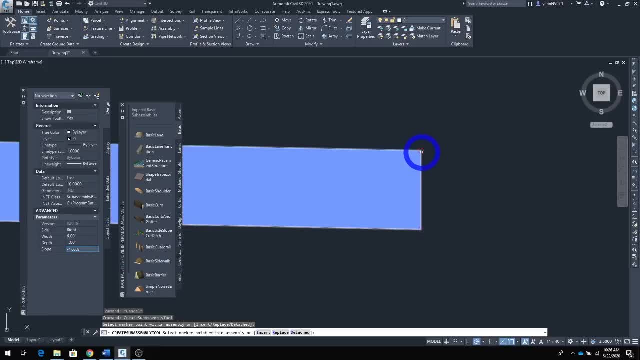 So we go ahead right here and click right there And there's our shoulder. Now we're done with the shoulders, Can put some curve, and then we can put some sidewalk. So if you can find curve back in the basic tab again, we go down as basic curve, or 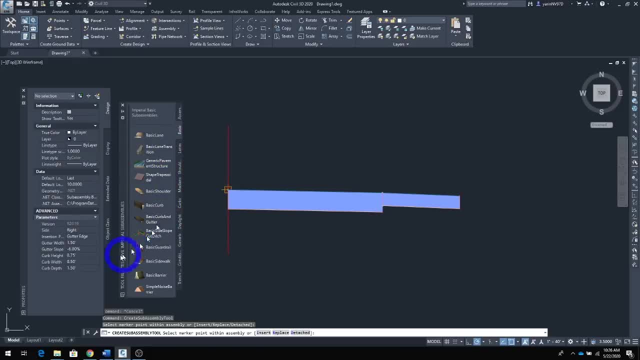 maybe have a curb and gutter. Okay, Click that And then you see on the right Side, Correct. Yeah, those information is good enough for me And come back in here and click right there And there's our curb right there also. 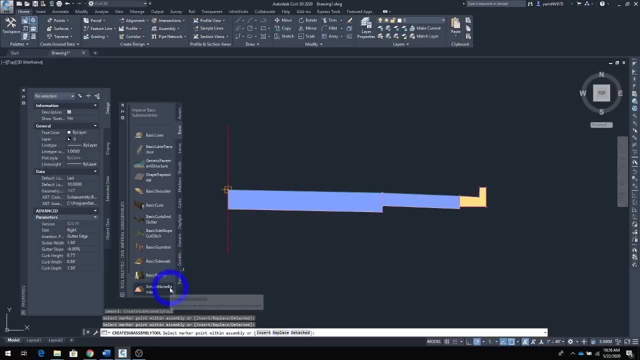 So now let's put a sidewalk next to it. Sidewalk- Where are you? Come back in here in our tool palette You can find sidewalk and we go basic sidewalk right there. We click on basic sidewalk on a property says six feet. 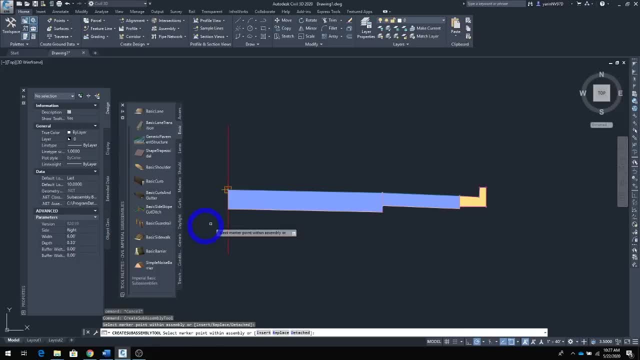 Six feet is good. That's the depth is all right, And let's do that, And we click our sidewalk. Start from right here at this point. Now we've got a sidewalk too. Now, when you finish this, you have to complete it. 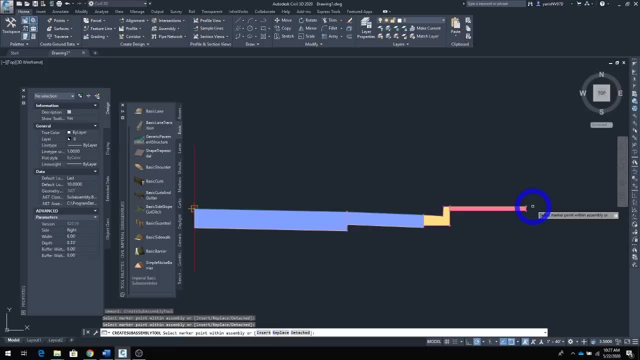 So daylight out the end of your section And that means you're connecting proposed grade to existing grade. So that's what daylight mean: We're going to go ahead and daylight this out and we're going to come back in a basic tool palette right here. 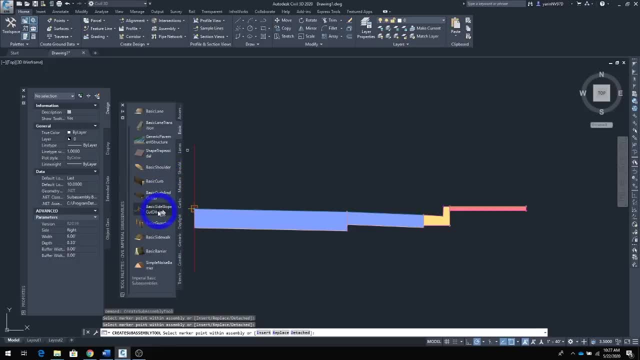 We look for right here, back slope and cut ditch, And you know that we talked about in the class what those are really a good way to look at. go take a look at the roadside design guide. They have a lot of good information there. 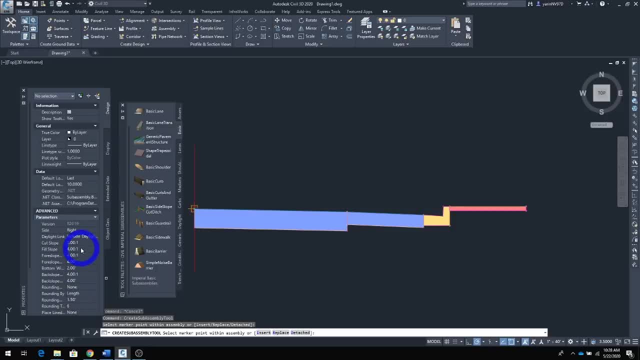 So now we go in here, They have everything right there. We want it, That's good, And go back in here, Click right there, There's our cut slope and fill slope. This program is so smart And a cut slope will put a ditch in for you. 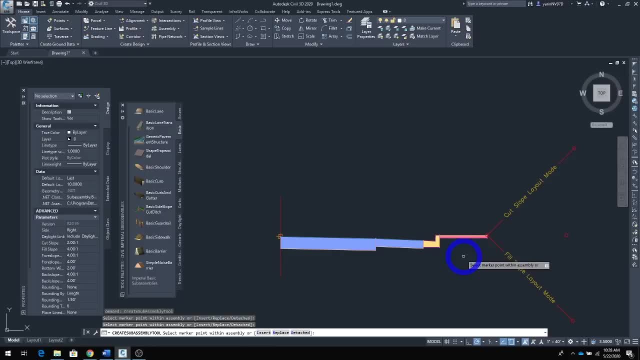 And again, you want more information. I will put that on Blackboard. It's a roadside design guide. We will cover that too anyway. So now we're good. This program is so smart, We can go ahead and do the left side. 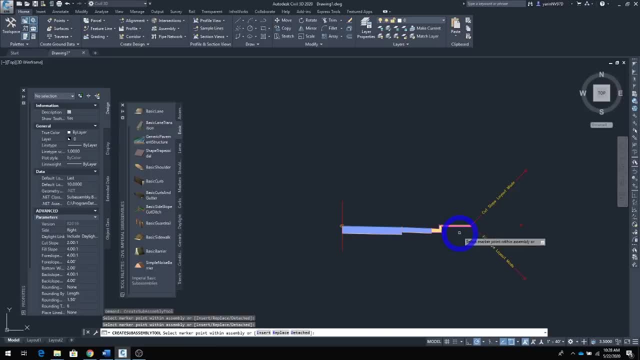 Or if we're going to know the left side, it's going to be the same thing. We can copy this and mirror it. Let's do it: Copy and mirror, Or you can. You can just go ahead and go to the left side. 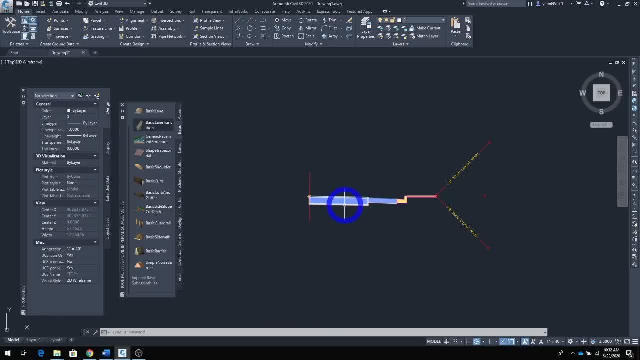 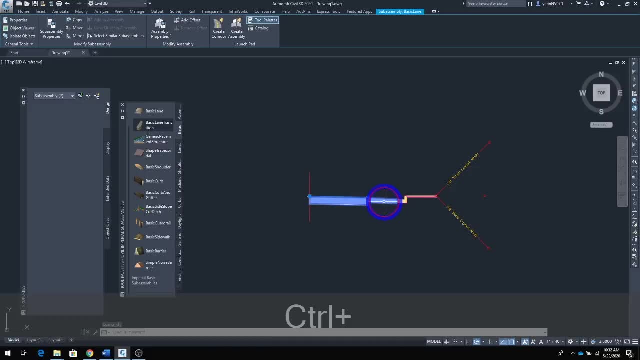 See if we can do this. Let's see if you can do this. Okay, click on this, Highlights it and hit control. Same one. Next, all of them. You can select all of them at one time and put them in this mode. 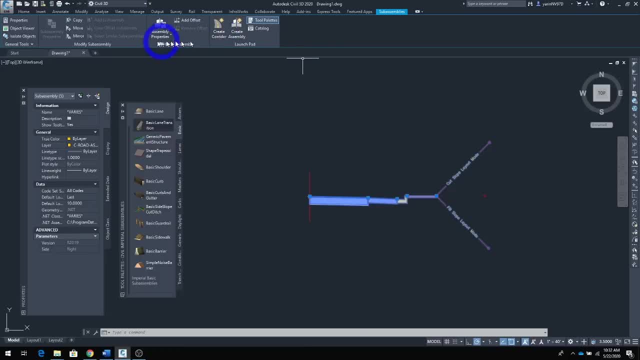 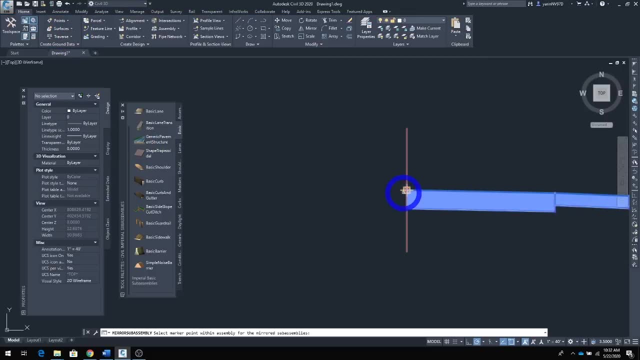 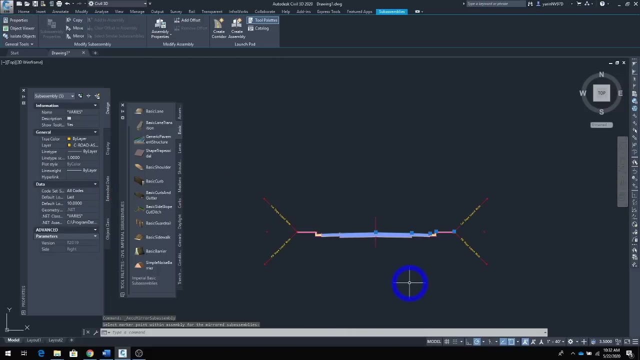 Once you do that, in the ribbon dialog box up here you can see an option called Mirror. Click on Mirror And then you come in here and mirror to this left side, And there it is. So now we've got them on both sides. 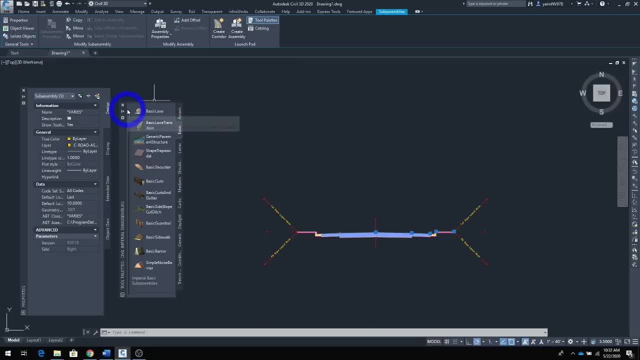 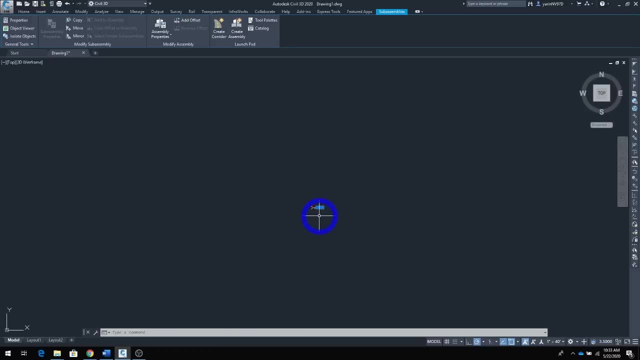 Okay, let's get rid of these. here We have more room, And I want to show this how small it is compared to there. it is right here. So what I want to do next? I want to go ahead and create a corridor. 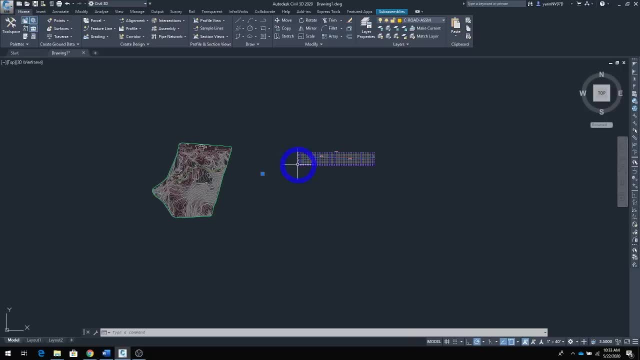 Go back to the home tab. right now I want to have a divide my screen so I can show it a little bit better. It's easier for me. So I'm going to go to view tab right here in the view tab I'm going to click the view configuration. 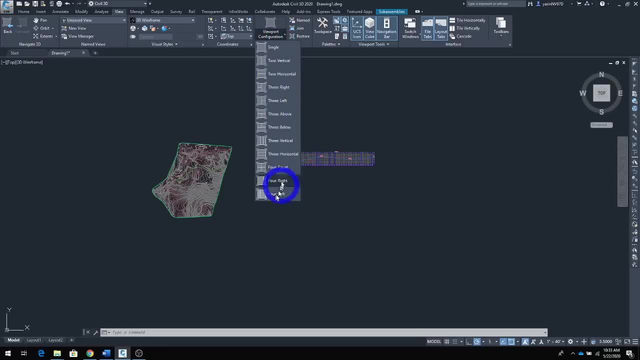 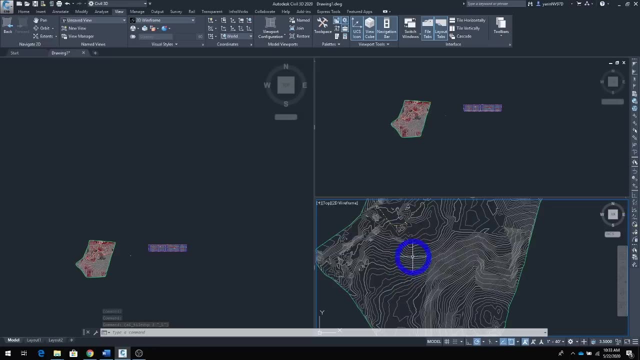 There's a drop down menu and you can do anything you want right here. Go right over three left. I will have three of them and I'm going to come in here first. I'm going to show my alignment. Okay, that's good. 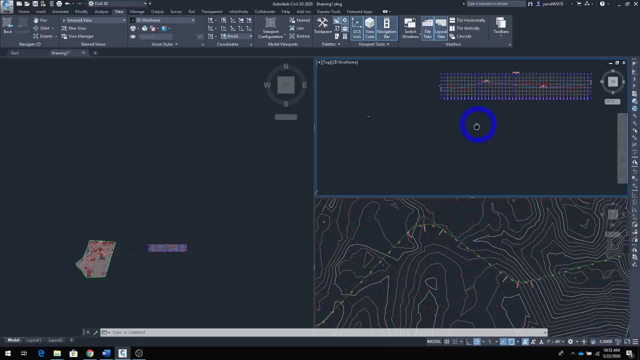 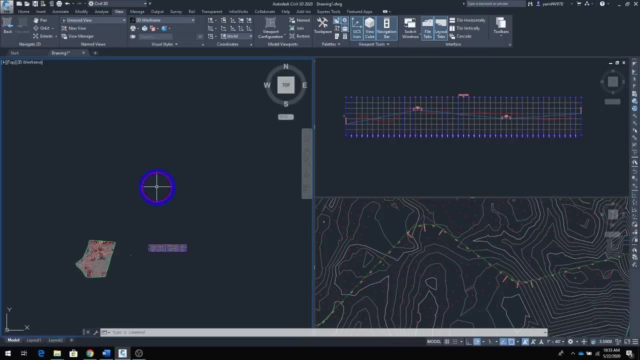 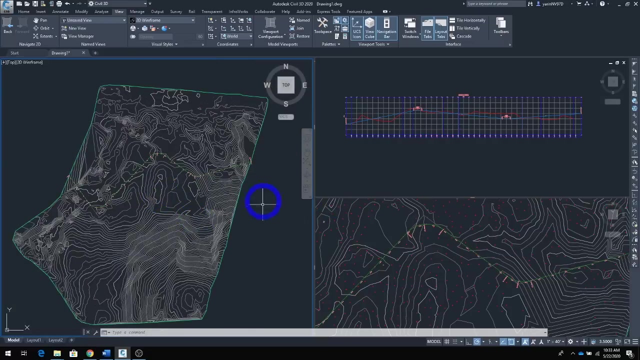 And then I want to show the profile in this view, All right, And in here, just oops. And here we're going to just show the alignment. There we go. So now we're going to go ahead and go back to the home tab. 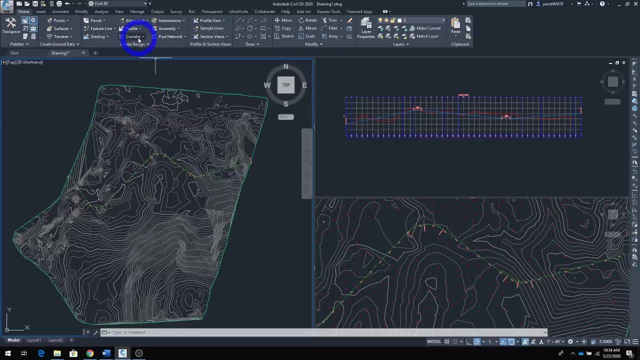 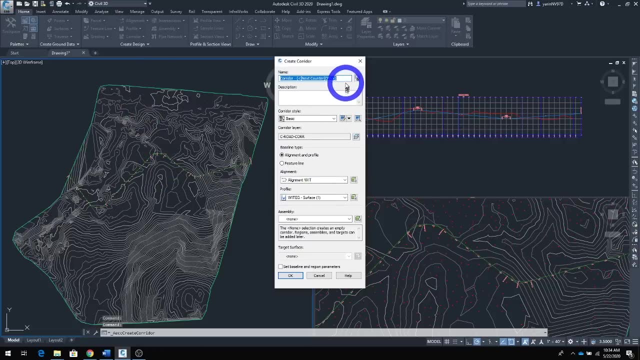 And from home tab you can see there's an option called corridor. You can click the corridor and hit corridor and a new window opens up And then the corridor- let's call it WIT Avenue- And the basic is good for this one. 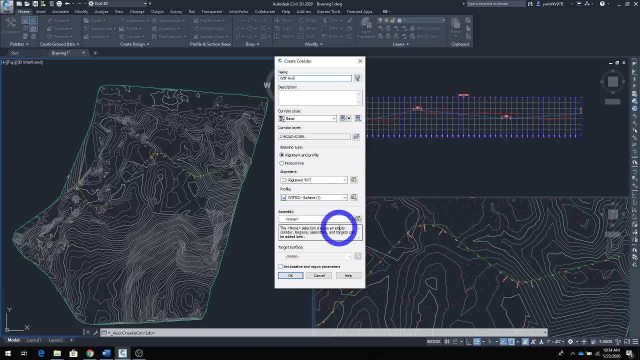 And you go down here It says these three options right here, Very important. So we're going to use WIT alignment. That's correct. If you click that here, then you click on the alignment is the same thing. So we know we have one alignment. 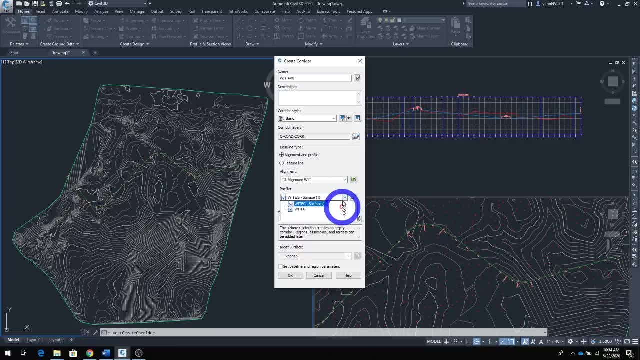 But in a profile view we have two of them. We click right here You can see two profiles. It says WIT EG Or WIT FG. FG is the one that finished grade, So we're going to go with that and assembly. 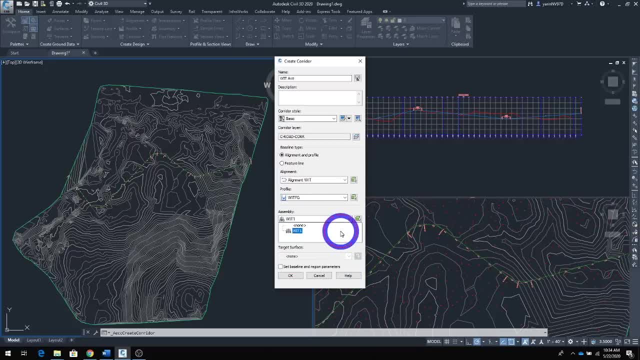 See what we have, for you Only have one, So we click on that which we have right there And then you go to the surface, You clip that, Keep that as none And make sure this box is unchecked right there And we're good to go.